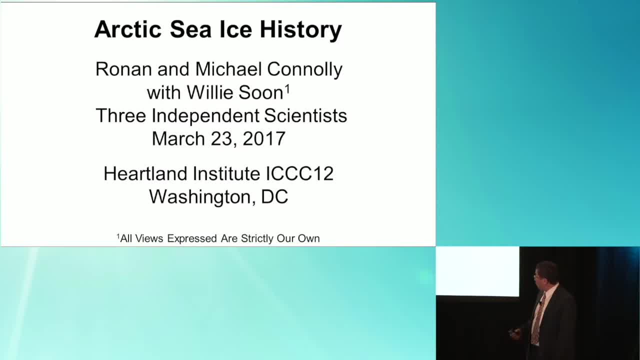 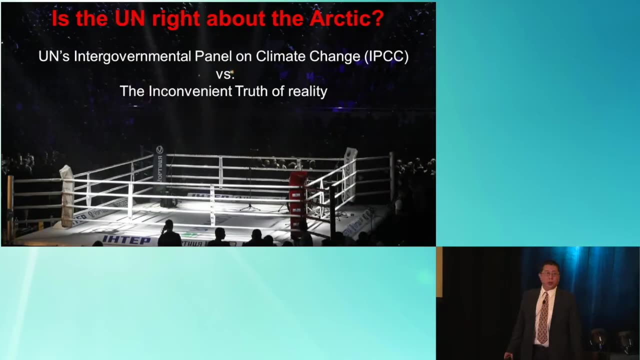 sea level, Arctic sea, ice history. This is really a work that is done of our own free will. We are truly, truly independent scientists, independent of fundings and all of that. So we're going to put UN under this boxing highlight. We really want to check whether 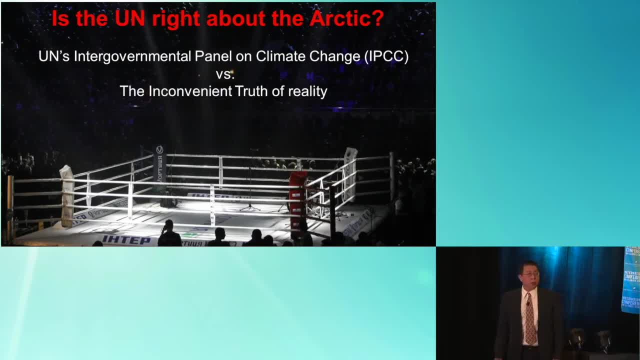 what all these statements that has been said about the Arctic, the climate and, of course, the sea ice, which is a key factors signature of Arctic region, the polar region, whether what has been said by the UN Intergovernmental Panel on Climate Change has any resemblance. 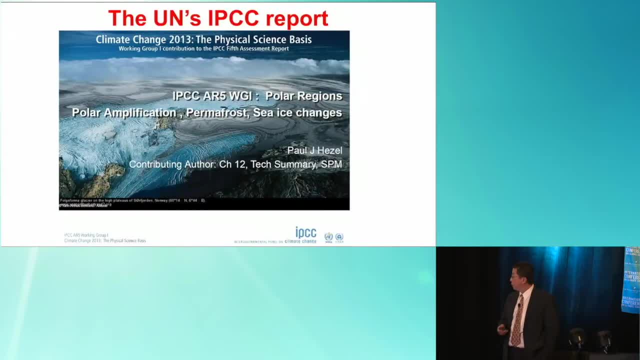 to the inconvenient truth of reality. So we'll start with that chapter from the AR5.. For those who are not familiar with AR5, it's the fifth assessment report. I hope they don't produce keep producing this. In fact, the sixth assessment is coming up, So we are going to examine what they've been said in. 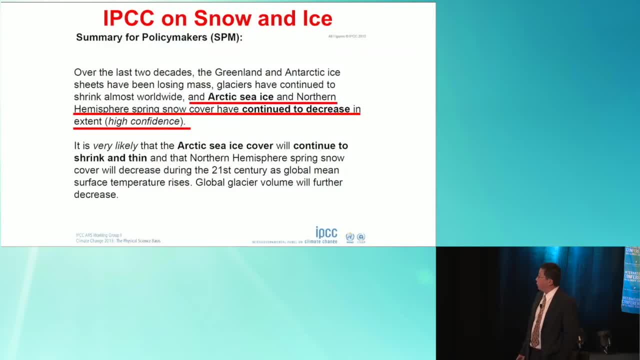 this particular report. So I will highlight for now two simple question or statement or claim that has been made by this report. The first thing is about Arctic sea ice and Northern Hemisphere spring snow cover have continued to decrease in extent And they say this is very high statistical confidence. So let's look at it First: spring snow ice disappearing. 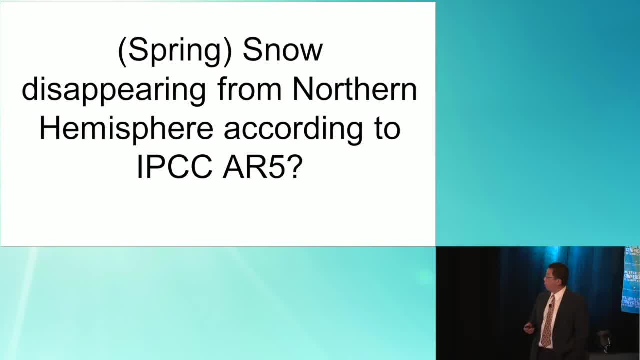 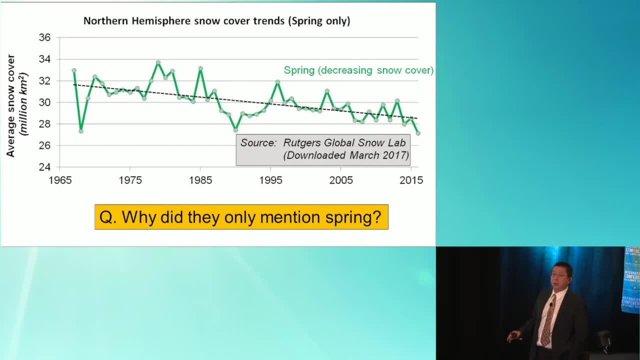 from Northern Hemisphere, according to IPCC AR5.. So how good is that statement? right Data shows 1965, since we have some satellite coverage, we can actually do a very good documentation of wide area so we can measure this particular changes over time. 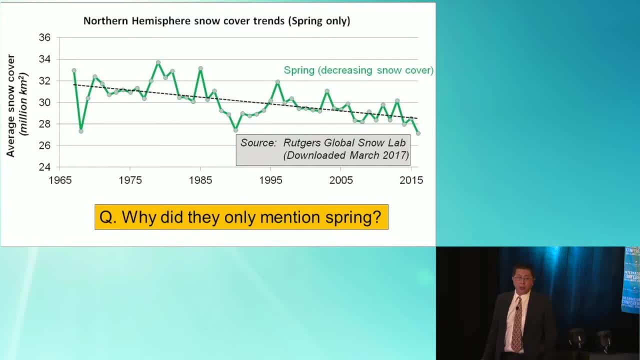 Indeed, the spring Northern Hemisphere ice snow cover has been decreasing. But I guess the key question that I highlight down there is: why did they mention only spring? I hope you all know the answer right. It's very simple. It's just simply because the snowfall. 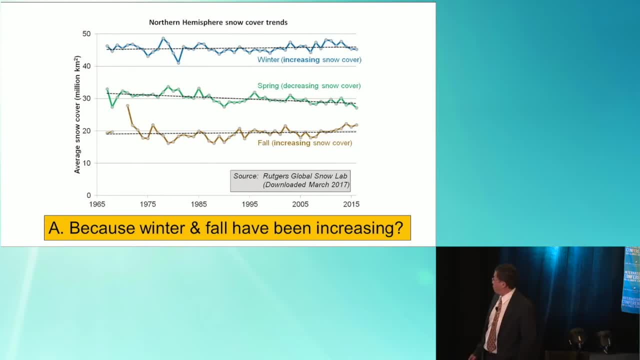 has been increasing and then the winter snowfall has been increasing. Too bad that I don't have time to explain why the spring snowfall is increasing. It's probably related to the increasing spring insolation, The changes over time period due to the orbital changes of the planet perturbing the Earth-Sun. 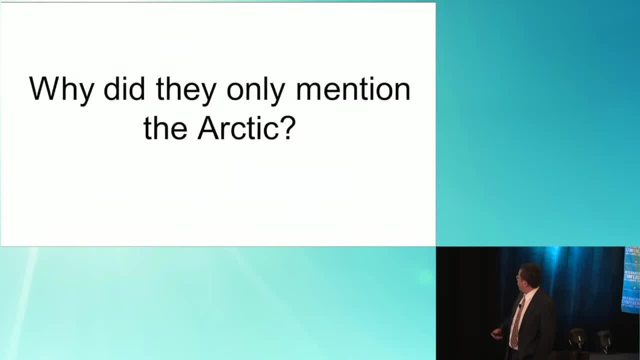 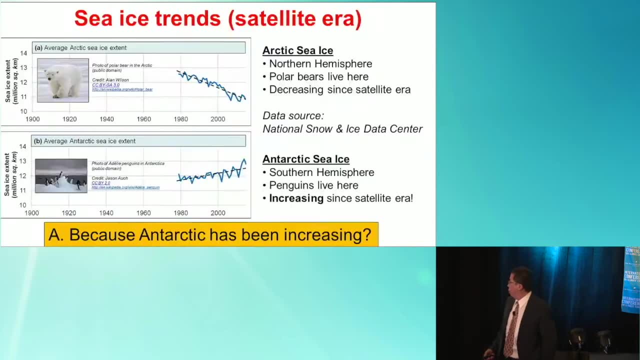 geometrical configuration. The second point is: why do they mention only the Arctic? Isn't that convenient? Arctic sea ice has been decreasing. Yes, we know it's been decreasing. Where is the data? The data is here On the top panel. you know where polar bears live. That's why we call Arctic. 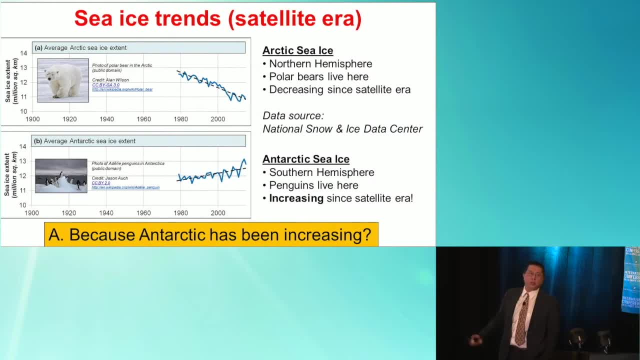 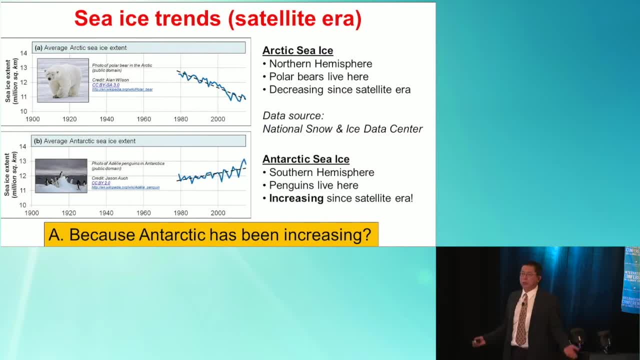 it. It doesn't make sense to only talk about the Arctic and then don't talk about the Antarctic, right. It is that kind of stuff that makes people really don't want to trust UNIPCC. I for one would never trust. Ask my son. independent of me, he won't agree with this. 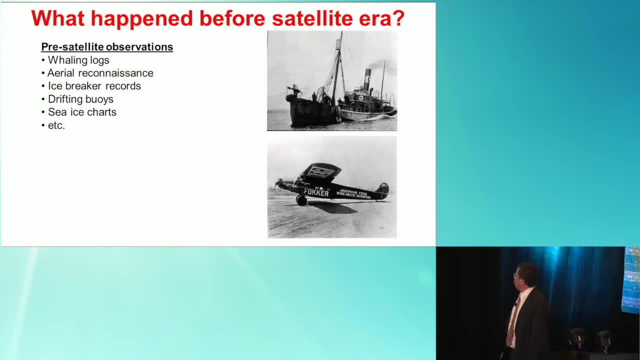 sort of statement. It's ridiculous. But what happened? Remember, this is based on satellite observation, but the key context about science is always: is that, okay, we have this measurement, but what is the error bar and what have we seen before? that sort of stuff. 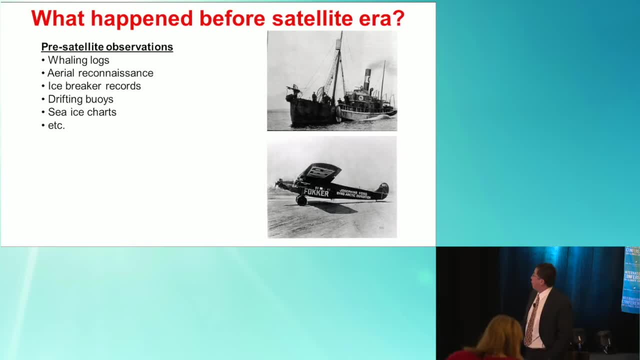 But before satellite era we really have very limited record. In this particular work that we're doing we went to really enormous amount of work looking into whaling locks, aerial reconnaissance, icebreaker record, you know. all this stuff, all this good stuff that at least give us a sense of reality. 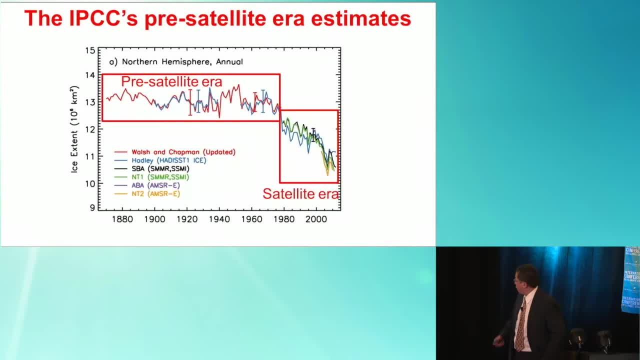 because we truly believe in database sort of discussion before we go anywhere else. So this is the way the IPCC report would present the result: The satellite era. we of course highlight for you to see that this is the big difference between satellite era, because the problem is that we really know that the climate changes, as Don has shown very well. 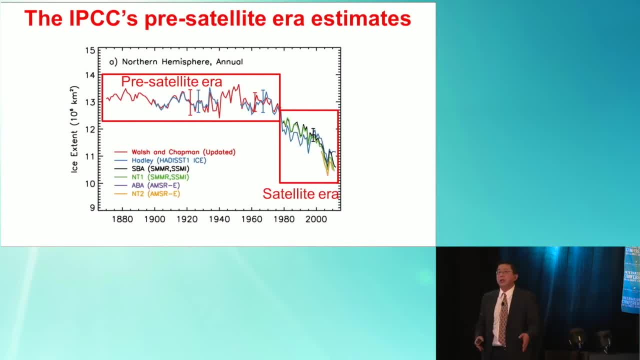 changes on the multi-decade of sand. You have warming, you have cooling in every 50 or 60 years or so, kind of oscillation. But look at the pre-satellite era, from 1900 or so to, let's say, 1970s. 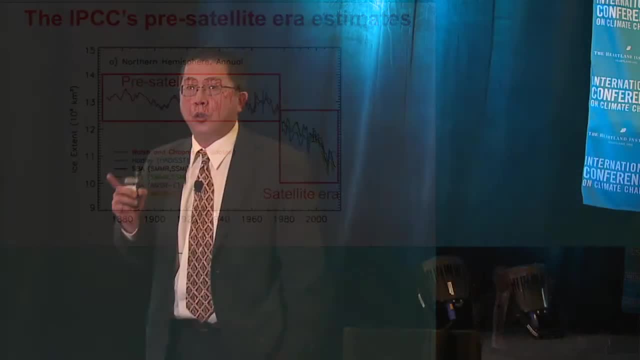 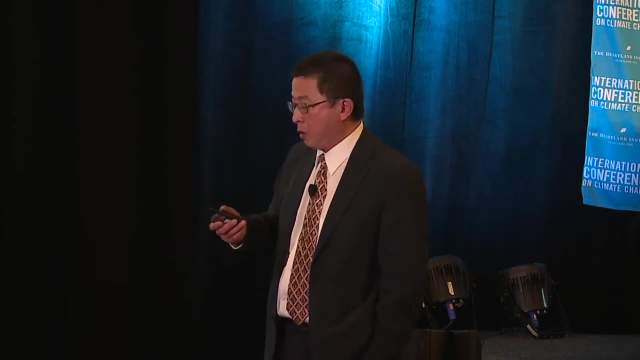 Kind of flat, isn't it? Plus that we know very well that from 45 to about 76 or so, there is a period, There is a period of cooling that is happening in the Arctic, But how come the sea ice data is so flat right? 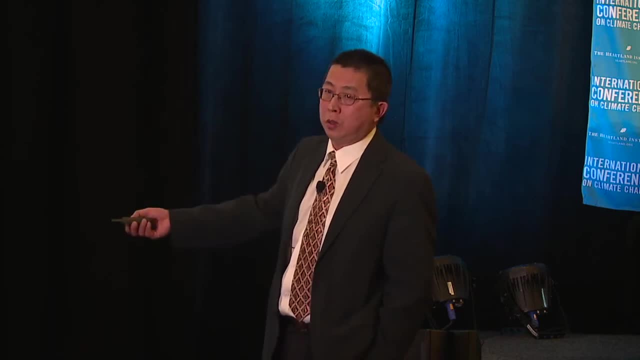 But this is the official record. This is why we are very suspicious of this result. so we went to and checked whether it's true or not, because science is about also verification- independent verification. Obviously, you know that we didn't come up with the same answer as them. 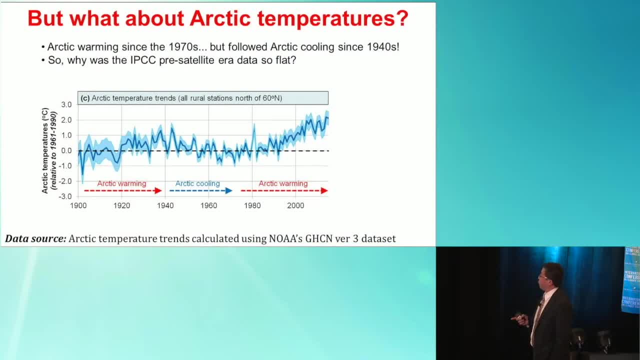 so I'll show you later. But we know that from Arctic temperature. by the way, information on sea ice is a lot harder to collect than at least the temperature, even though it is imperfect. but we have a good sense. We have a good sense of Arctic temperature covering about 100,. 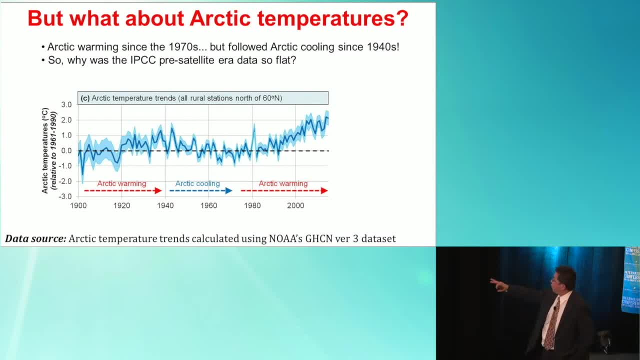 you know, 150 years or so over the Arctic. You can see that from 1900 to about 1940, you have a warming period and then 1940 to the 70s or so is cooling and then Arctic warming again. okay, 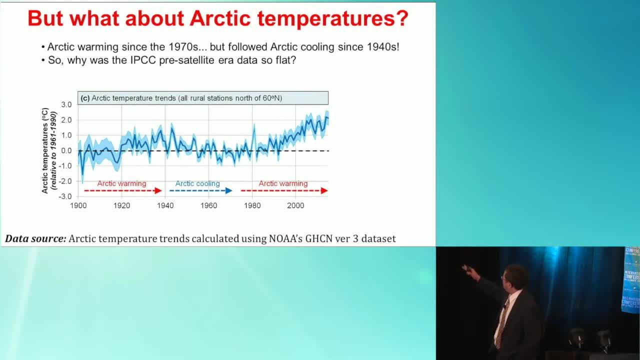 But the key question is: yeah, indeed, even if you have the warming, from the 70s the Arctic sea ice has been decreasing, but we know that it follows a period of cooling, So where is the evidence for that? That sea ice is increasing. actually it's supposed to increase. 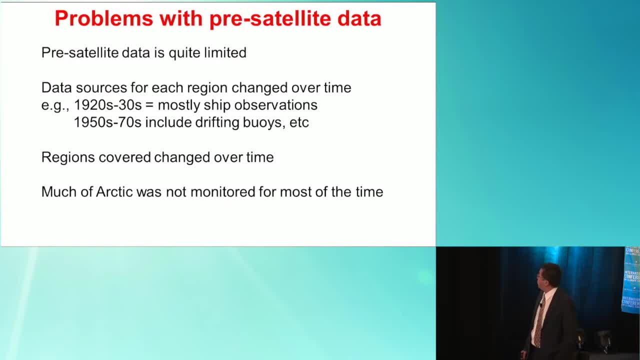 So this is the three kind of major problem with pre-satellite data. The first one is actually the data sources for each region is changing over time. So for example, 20s and 30s, you have mostly the ship observation. 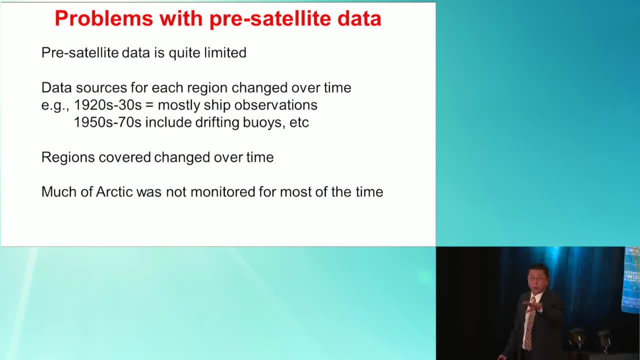 From the 50s to 70s. you have the really in situ, the buoy, which is really also very key in giving us real information, And then you have region that cover the change over time. okay, Finally, really the serious problem is that most of the Arctic 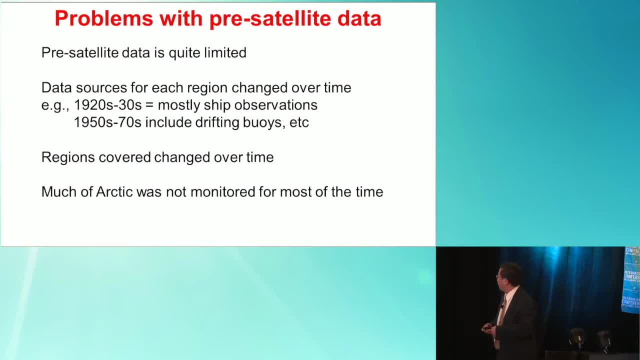 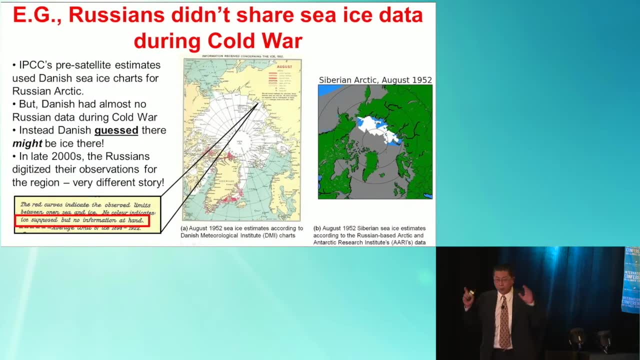 was not observed at all. Nobody has the real data to look at these things, So it's imperfect, but here's what we come up with. But we give one example now on this problem from IPCC report. okay, On your left there is basically so-called sea ice map that is produced by the Danish. 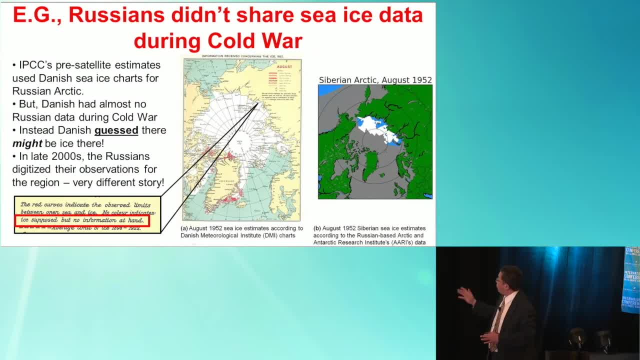 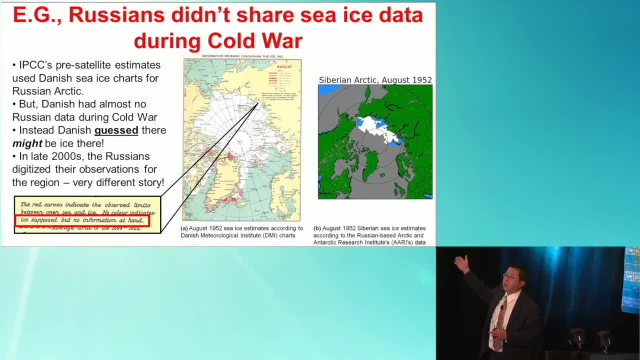 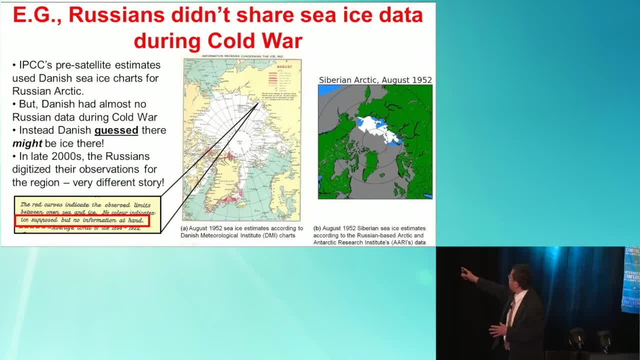 So they are only guessing. And then, ever since then, because those are the Russian sector, those are the Chukchi Sea and the East Siberian Sea, and you look at the actual data, that the Russian just released, the data, and we have gotten those data from those great people from St Petersburg and 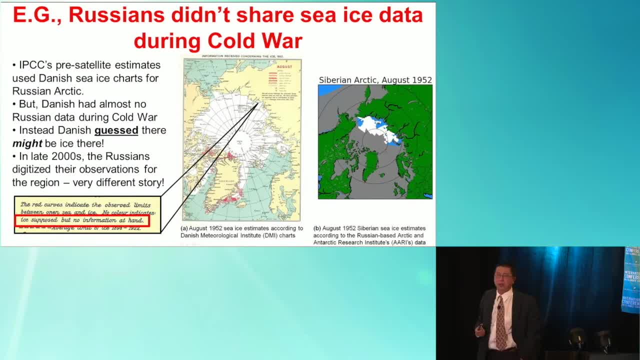 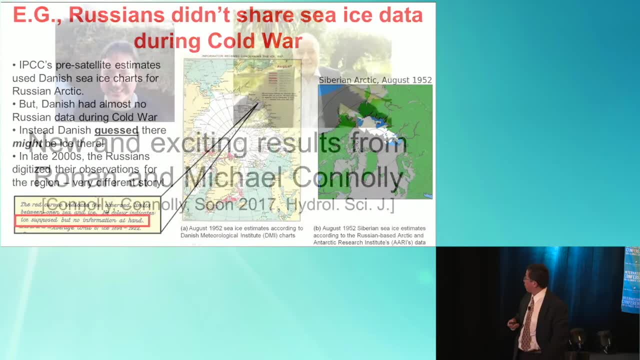 they're showing the data like that. You can see what a mismatch of information. okay, Over-exaggeration. Over-exaggeration of the sea ice, actually pre-satellite era, showing as if that now the change would be very dramatic. 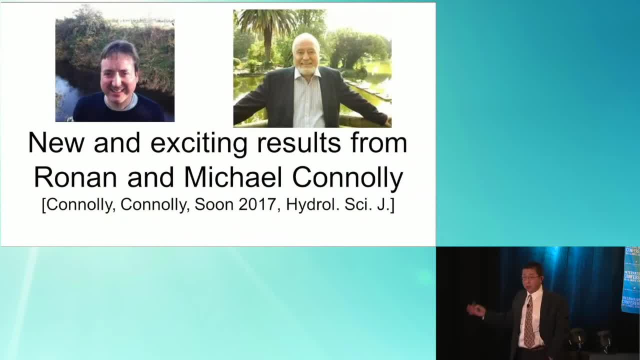 So this is a new work. The paper is already accepted. it's in the press, so please ask us for the paper in case you want to read in more detail. So no way I can cover this in 15 or 20 minutes. 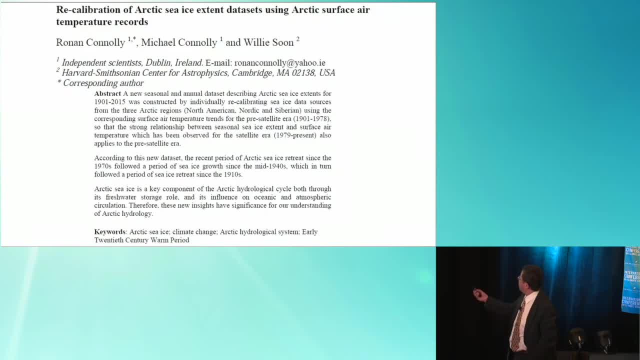 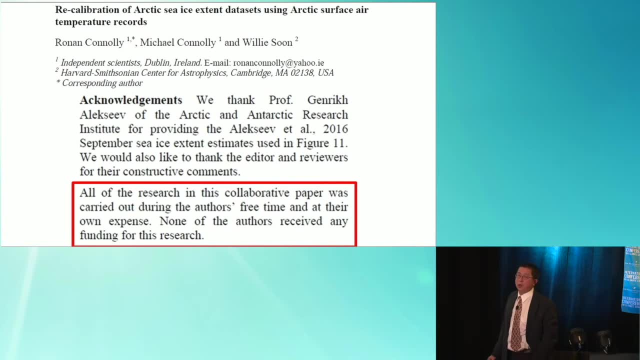 These are Ronan, this is Michael And this is the paper. Don't read the abstract just to show you that it is a work that has been accepted for publication, But a very important point that I want to make which bothers me a lot. 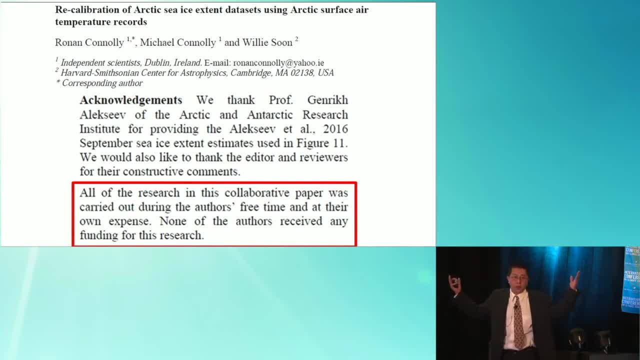 Is that this work? I'm not even supposed to do it As a scientist. Okay, It's not an official work, So it's doing it under my own free time, under my own volunteer. no expense was covered by anyone or anybody. 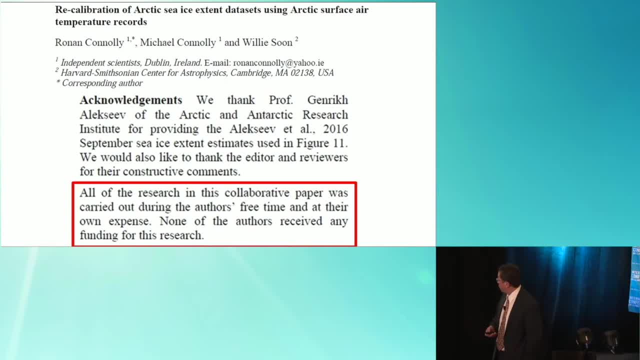 And we just do it our own fun for learning about the science. Okay, That's the only. that's the big point. To try to make the point that you know you don't really need big money to do good quality science. You don't need all these endless charades of asking for funding and all this circus. 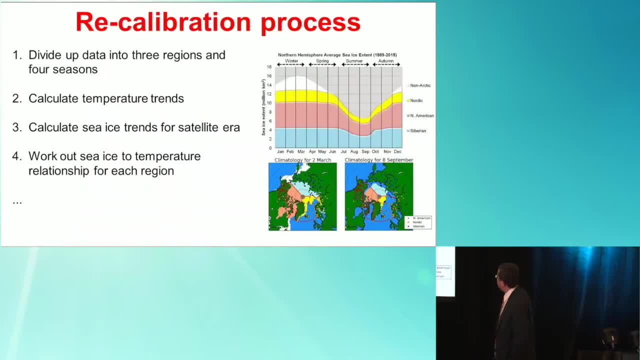 about money, this money, that Okay. So for this real work, these are the steps. It's very simple really, But the main point I want to point you is that, for Arctic sea ice, look at the seasonality, how you define it. 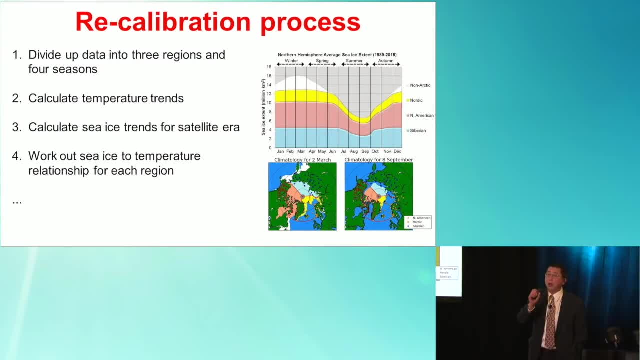 For summer, it's not. it's not June, July, August, it's actually July, August and September: sea ice. You have to account for the real climatology, What happened there, So you really have to be really careful. 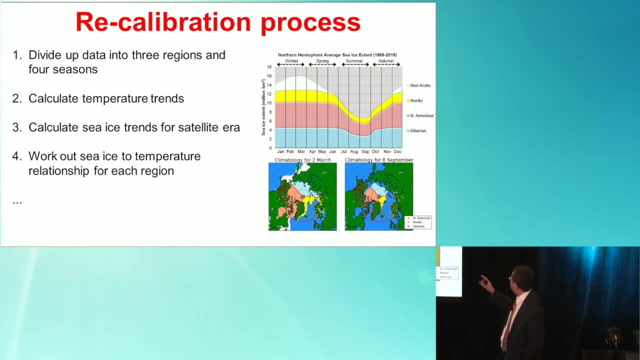 So what we did is that we divide the data into three regions. So we have the North American region and then the Siberian, the Russian region. And then we divide the data into three regions. So we have the North American region and then the Siberian, the Russian region. 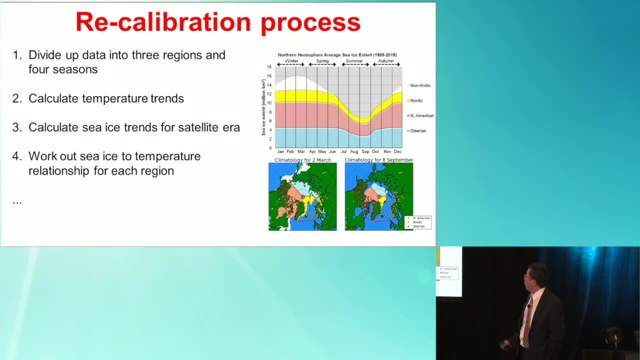 And then we divide the data into three regions, And then we have the European region. right? We actually use the information from temperature data. We calculate the temperature trend, We divide into three regions and four seasons, And then we get the sea ice data, the accurate sea ice data from the satellite era, since 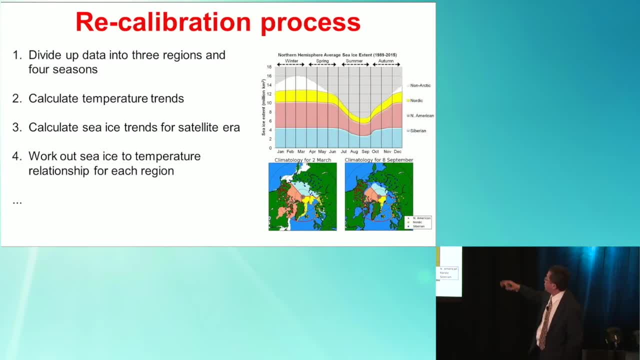 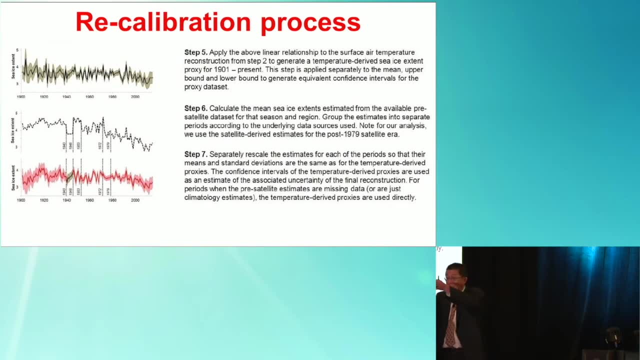 1978 or so, And then we work out the relationship between sea ice and temperature for every region And then- don't read into this- Essentially we use the temperature, the calibration that we have for this period, And then we use the temperature to bring back from to 1900.. 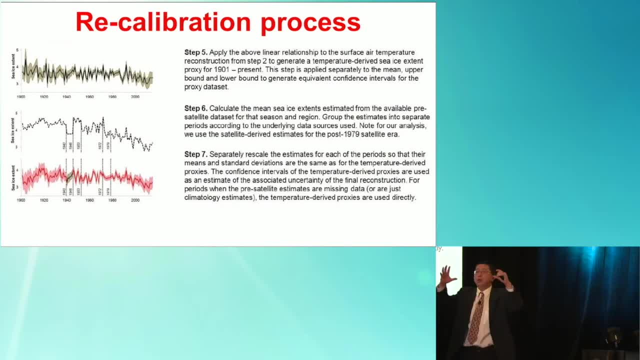 And then the key step is step six. We use all that is available of the sea ice information to check the mean and the variance, to try to really adjust it properly with respect to what is actually known from the temperature- calibrated sea ice, And then, finally, we rescale everything. 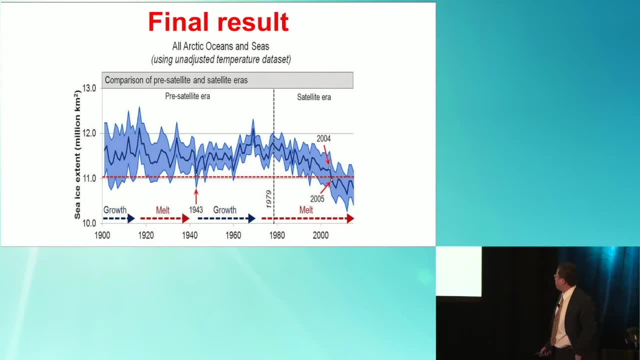 Please read in detail. This is a very careful work. This is the final result. So what we are able to show is that, yes, indeed, the satellite era, because we use the best data from satellite, you have melting, But the period of growth from 43 to 100 years. 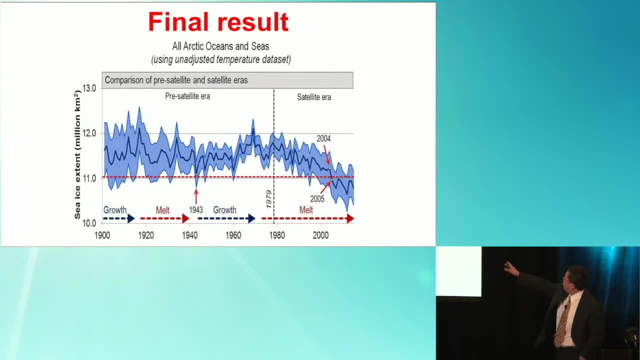 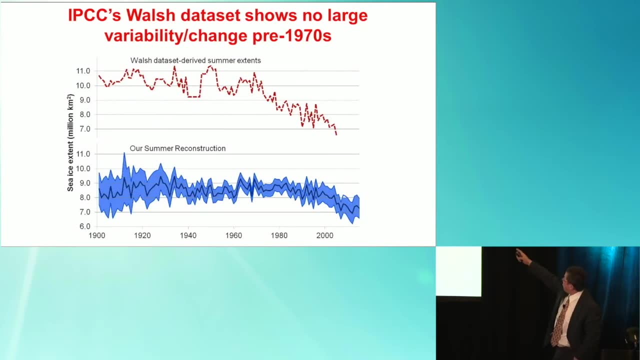 The period from 43 to 70 is real, it's actually happening. And then you also have all this up and down, right. And then if you compare with the summer extent of the IPCC approved result, you will see that the pre-satellite era is pretty flat. 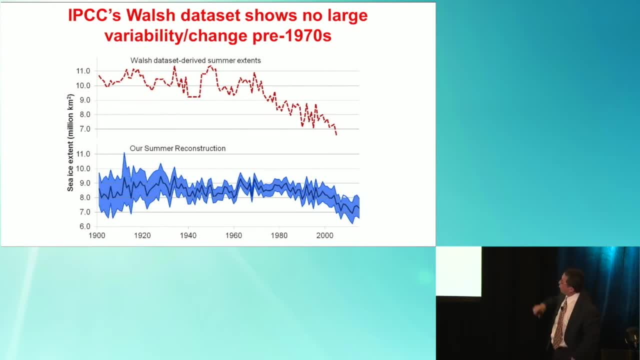 And plus that they never show the actually sea ice increasing in the 40s and the 70s And this is our summer reconstruction result. If you compare to that, I don't think it's too drastic. what is being changed now compared to the past period? 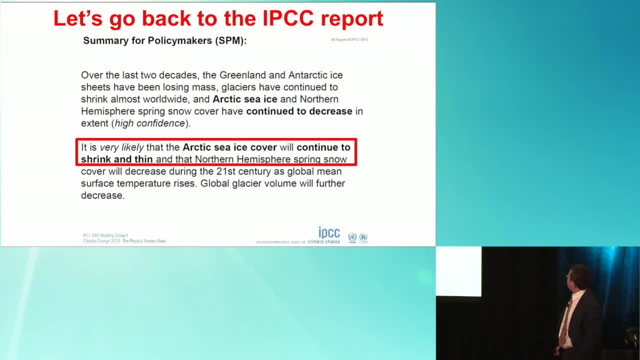 And let's look at this. Okay, Let's look back a little. another question, which is, of course, the IPCC claim. oh, if we don't do something about this, atmospheric CO2.. By the way, atmospheric CO2,, here it is. 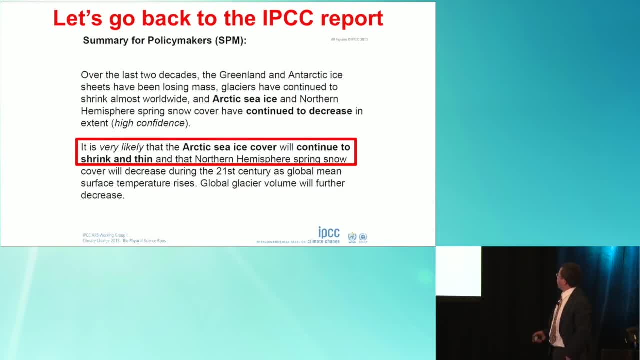 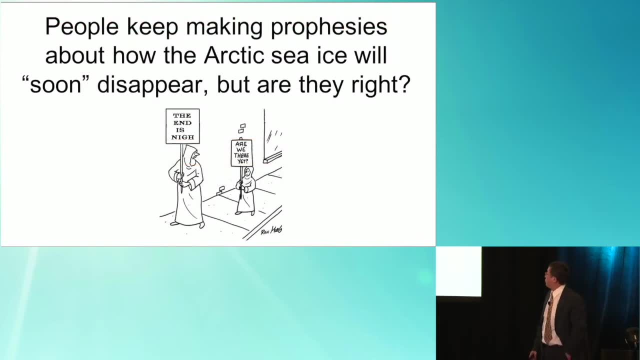 Arctic sea ice is continuing to shrink and thin in the northern hemisphere. You know that these are all purely based on computer model And they really been making this sort of prophecy about Arctic sea ice disappearing. Should we keep saying this? They say it will soon disappear. 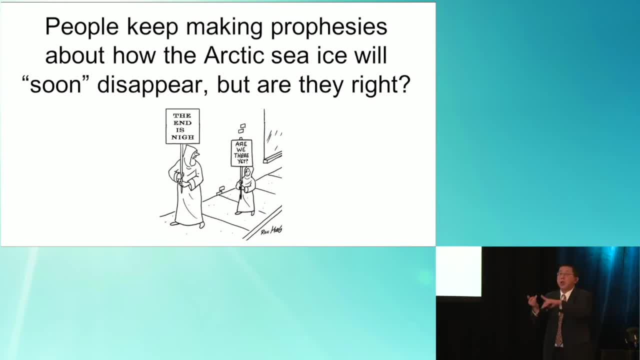 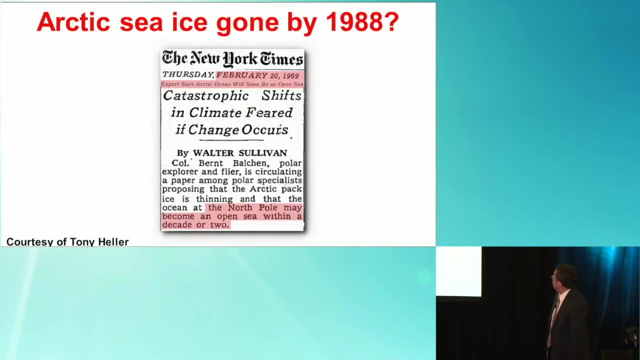 You have seen report from 2016,. it will disappear by 2016,, 2014,, 2012,, 2013,, 2008,. and then, finally, our good friend Tony Heller. one of these free, independent maverick, independent maverick. 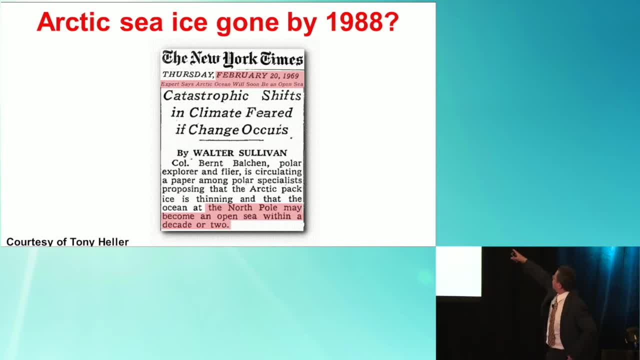 who actually also have known funding for this kind of work. He actually found this report from the fake news headquarter New York Times showing you that the claim of Arctic sea ice will be gone by 1988. It's really beyond belief. 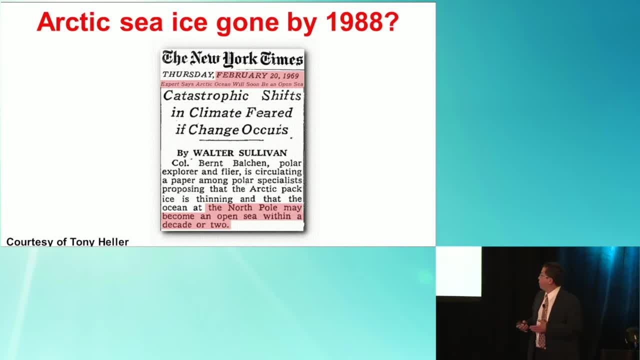 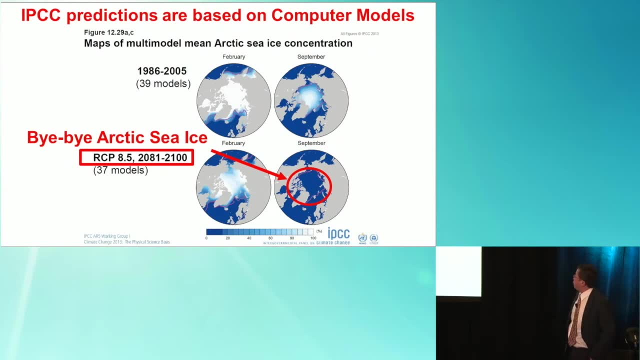 You know You keep believing in this sort of stuff. you know That it's not happening and yet we still believe that these people have any credibility of making any claims. And here's the way the IPCC wants to show you from, let's say, the observation period. 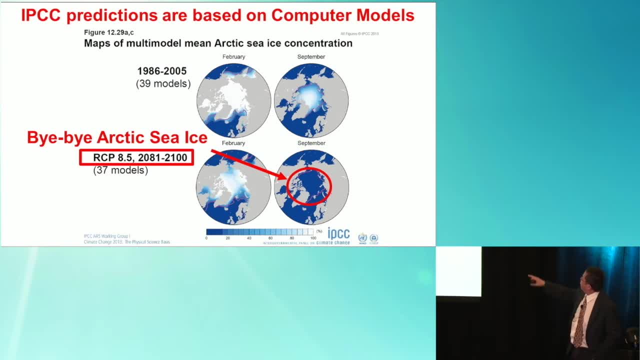 they show you: oh, this is so many models, we're producing this. and then by 2100, the scenario, by the way, is very extreme for the rise of atmospheric carbon dioxide, because they believe that the human population by 2100 will be 12 billion people. 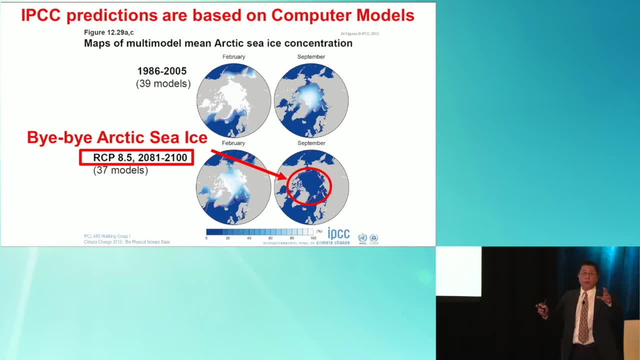 And then the atmospheric carbon dioxide of the equivalents. if you add methane and all this stuff will be almost 1300 parts per million, which is quite a lot. So sea ice bye-bye. But if you really want to believe in results, this result, I give you a little caution. 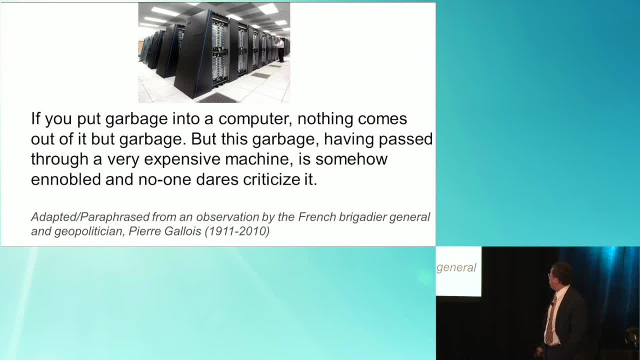 Since we have our French, our realist friends here. this is actually a quote from Pierre Gallois, which is the well-known father of the atomic bomb of the French people, And he says that if you put garbage into a computer, nothing comes out of it. 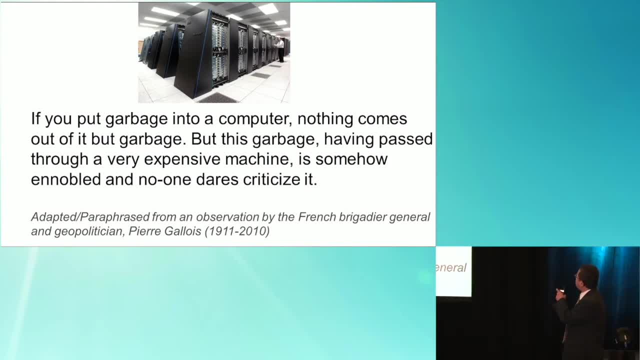 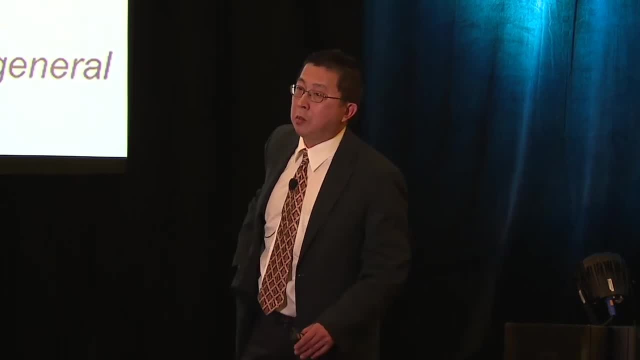 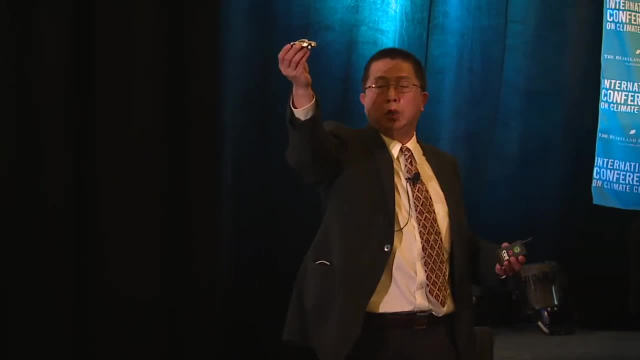 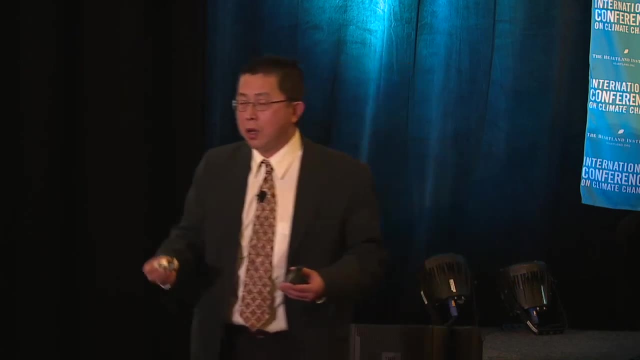 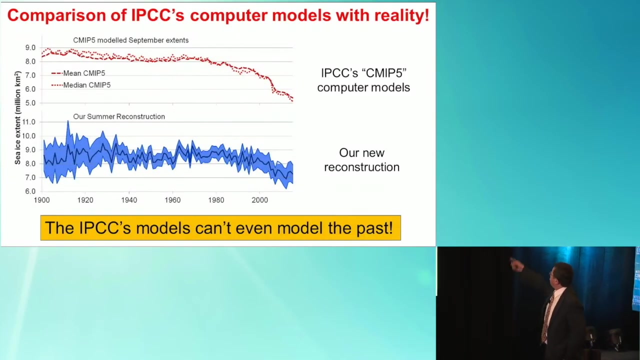 This is a lot, lot better to say this. IPCC want to tell you that this is a truck. This is a truck. Okay, This is not a model. Thank you, frankly, If you think, look at the computer model, This is what they produce. 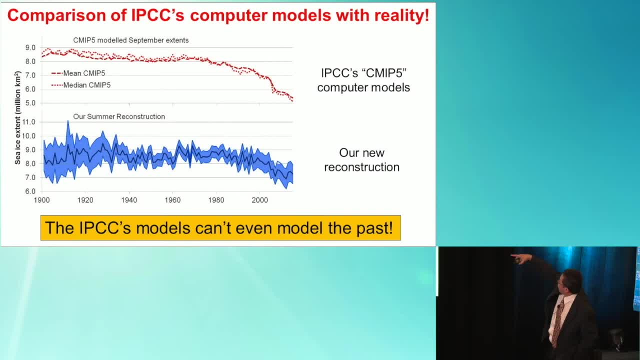 It's decreasing. This is our reconstruction. They basically are very flat from those periods and then saying that, oh, CO2 come along, it's going to decrease. But I truly believe that this is really really a natural kind of variability, even including 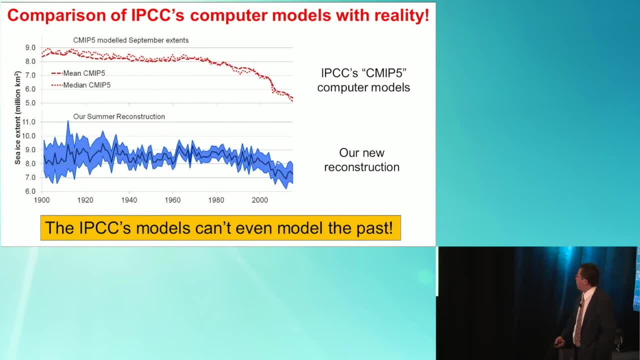 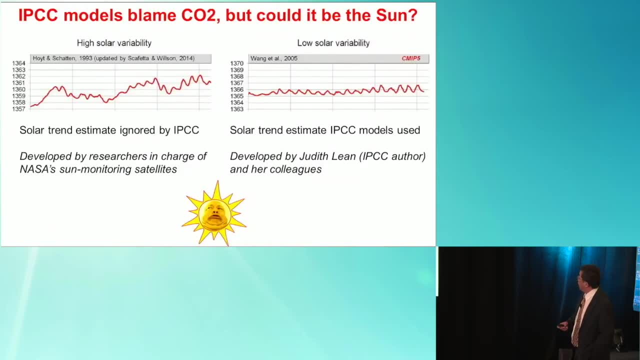 what we observe by now, 2016.. There's just no way you can make that claim. Yeah, it's the CO2 that did it right? There's a mother in the room And then, finally, if IPCC blames CO2, what is it that could do it? 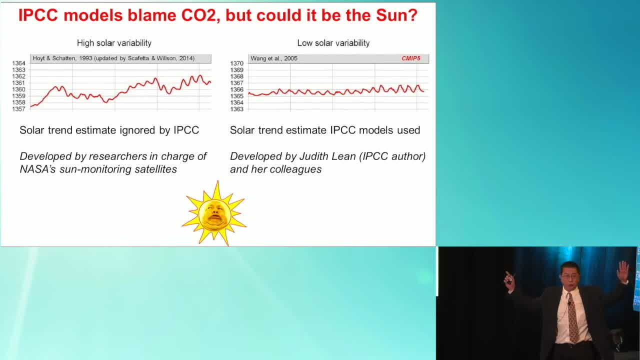 Could it be the sun? That's the question For this. for those full disclosure again, I just wanted to study science, okay? So in terms of solar variability, you can see I happen to choose to use that curve from the left. 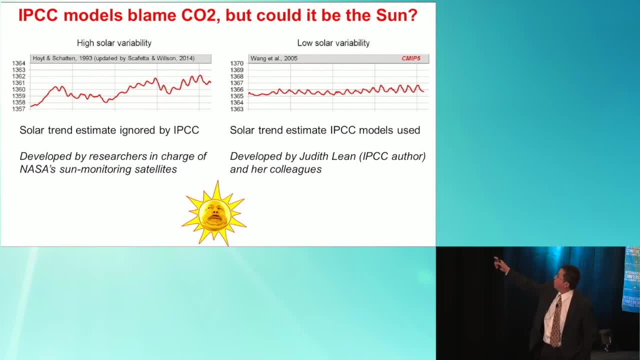 And then IPCC always promoted this particular curve and never, ever discuss why the other curve could be wrong or right. okay, It's always promoting this because they just want to believe in this particular people. And I show you now the results that we can produce with the Arctic sea, ice, Arctic surface. 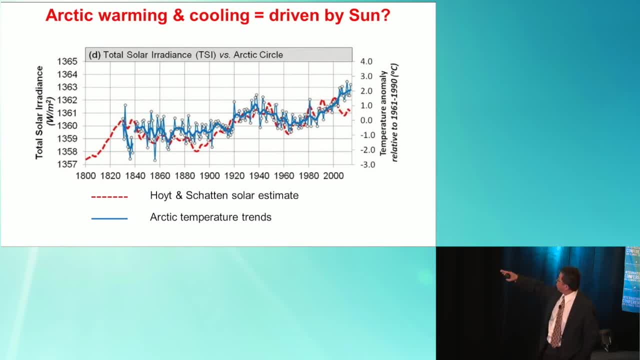 temperature. This is the paper that has been published. The blue curve is the temperature And then the red curve is actually the solar irradiance changes over time. okay, I think the fit is pretty good And this paper has been peer-reviewed and published. 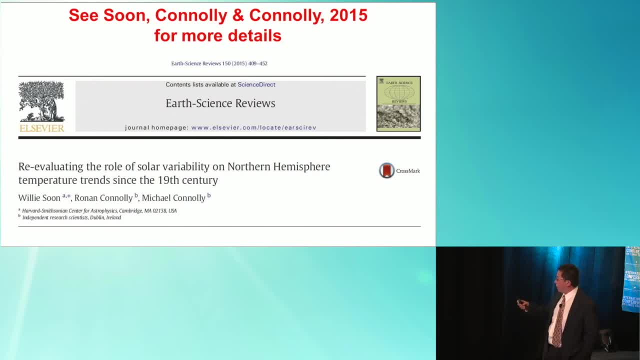 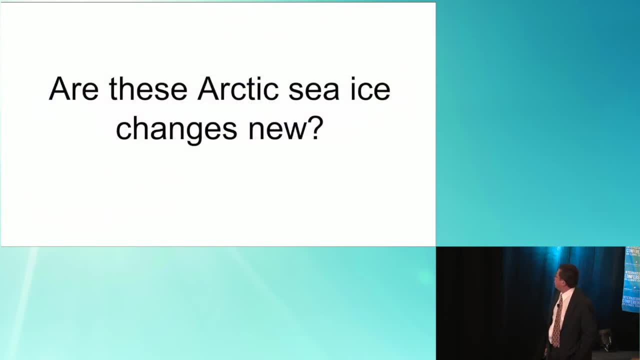 We published this just a year ago, So I hope everybody. if you have more questions, please ask me, or Ronan and Michael for reading. But are these Arctic sea ice changes really new? okay, That's another question that I want to answer before I finish. 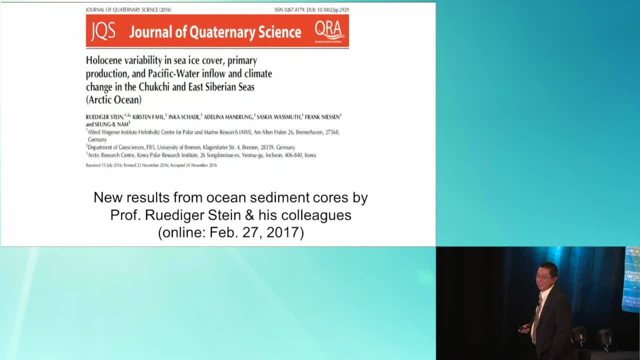 I'm almost done, Please don't keep flushing me- And it's based on a paper from Germany, Professor Rudiger Stein. I have already contacted them. This is actually a very, very good study that just came out about. you can see three weeks. 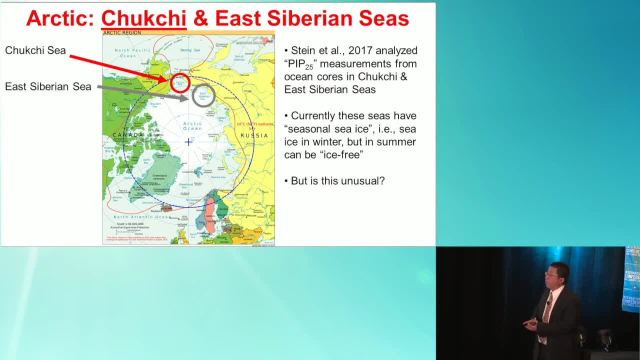 ago And what they are able to do is basically collected this ocean sediment by around the Chukchi Sea and East Siberian Sea region. I'm going to show only the result from Chukchi Sea. This is a very clever technique. It's actually plankton studying plankton. 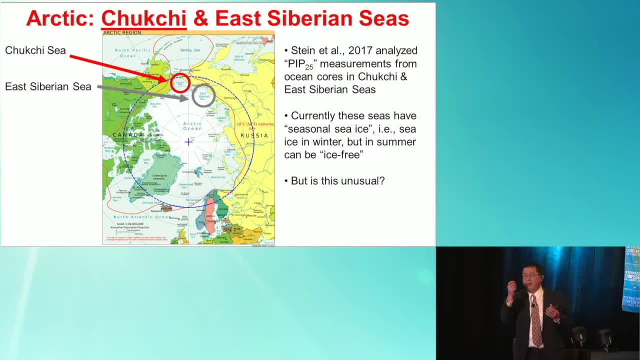 And you study a very special biomarker. It's from a fat, you know lipid form. It's called ice proxy, 25 carbons. okay, It's a very, very clever technique So they can measure it and it's kind of unique. 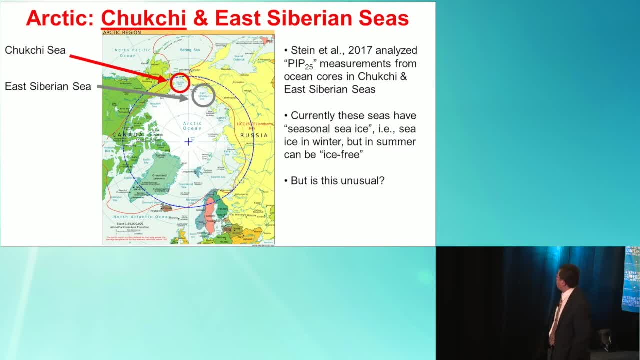 So it's very good work that's been going on. So, despite all the problems, I think we do have some interesting work. So they produced this new paper. Currently around the area you have basically seasonal sea ice. Seasonal sea ice just means that you have sea ice in the winter and then summer when 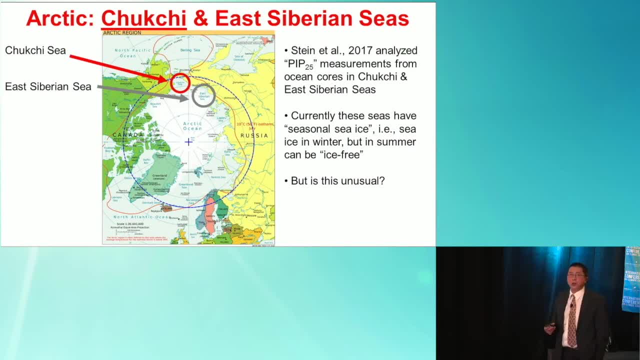 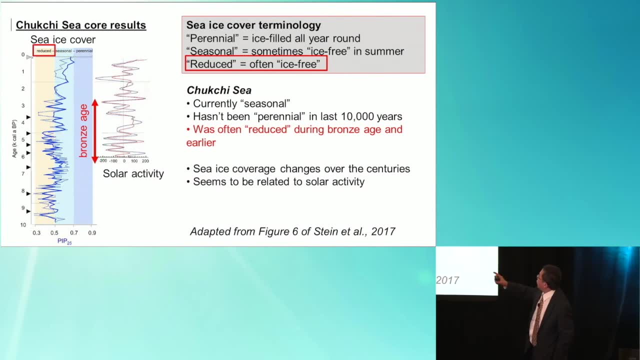 it's warm. when it's extremely warm, you'll be ice-free. But is this unusual? I hope you know the punchline For Chukchi Sea. sorry for the graph, but it shows you that you basically can have three categories of sea ice. 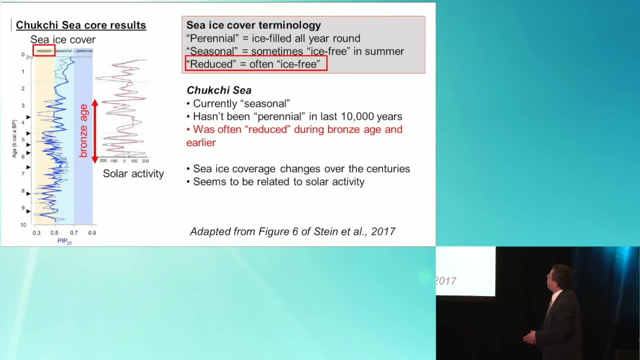 One is basically the reduced, which is actually often ice-free. You can see large part of the Holocene 10,000 years ago, until 5,000, 6,000 years ago, It's always ice-free, okay. And then you have the perennial extreme, which is the sea. ice is filled all year round. 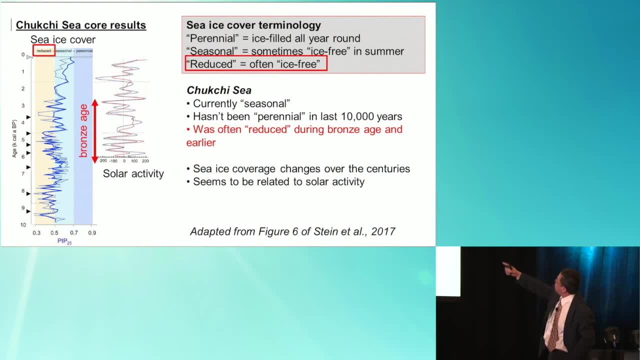 So for this region we have never seen it. For now we're basically mostly seasonal sea ice, So you can see that the sea ice actually hasn't been perennial for the last 10,000 years and it's often reduced during the Bronze Age and earlier right. 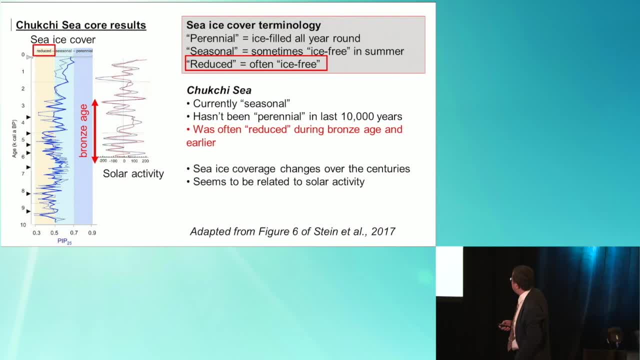 The Bronze Age is about 3,000 BC to about 500 BC or so, And the sea ice coverage changes over a century timescale and it seems to have relationship with solar activity, as shown by Professor Stein. So I'm done now. 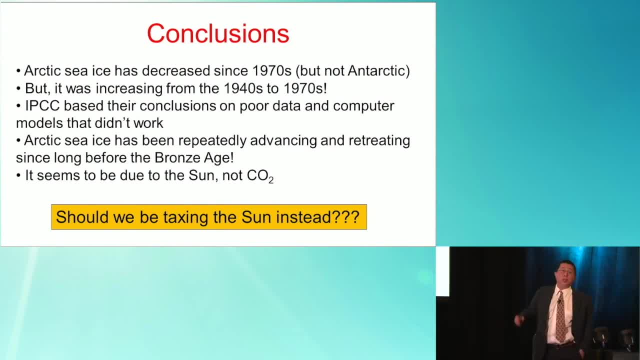 The question is: Arctic sea ice indeed has been decreased since 1970.. But the key point is: simultaneously, Antarctic sea ice is increasing. We really need to answer the question instead of just saying, oh, looking at just specific evidence that we found CO2.. 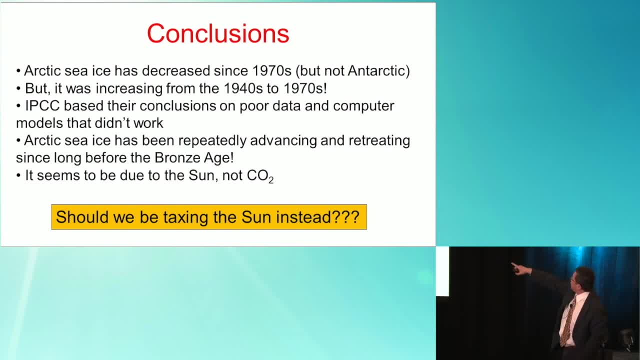 Obviously it's not CO2 doing that. Then you can see that it was increasing from 1940 to 1970.. Can IPCC try to explain that with rising CO2? Then you can see that IPCC's conclusion, especially those future projections- another you know. 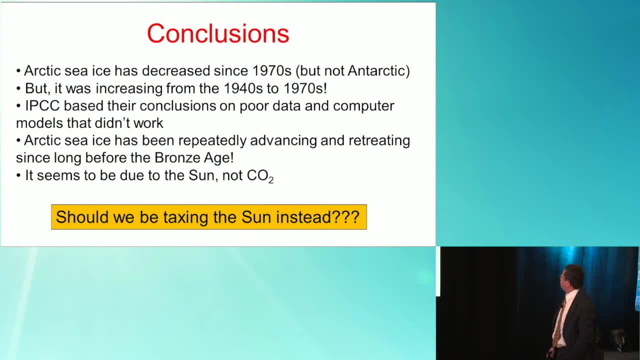 85 years from now is based on computer models. I mean those, Those things, I mean as good as my modeling work, right, So it's not good, It's really not good work at all. And then, finally, Arctic sea: ice has been repeatedly advancing and retreating long ago. 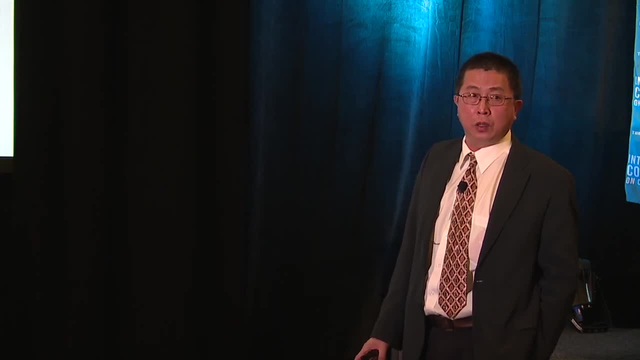 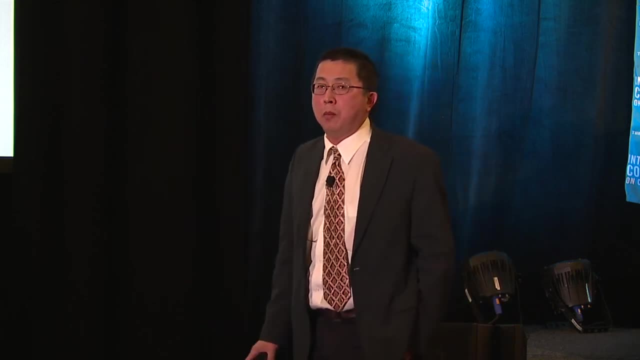 since before the Bronze Age. Was anybody driving SUV then? So I also conclude that from all that I know, I look into this. I mean it's really that maybe related to the sun, although you know we don't come here to bang our chest- that 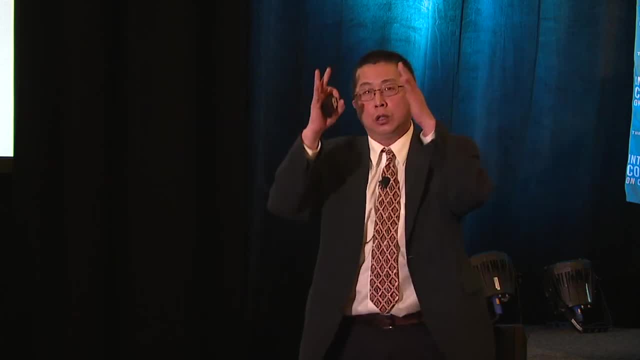 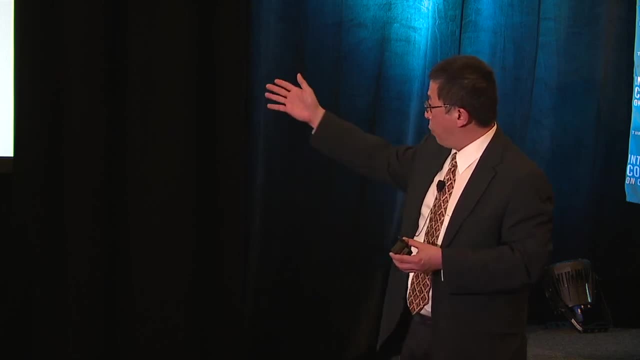 I'm so smart that I found the sun to be doing that. Science is a continual journey of keep testing, Keeping and retesting your ideas and your hypotheses and based on what the data is available. So I propose that IPCC should start taxing the sun if they don't like this idea. Thank you.